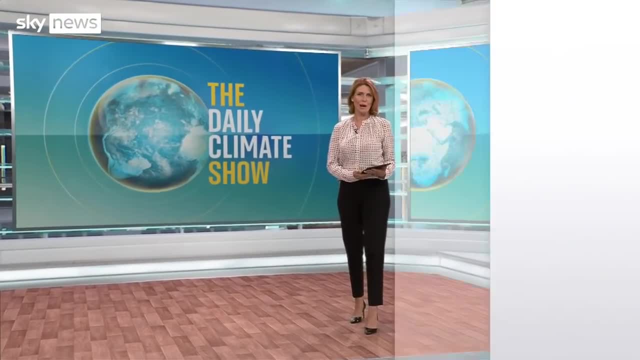 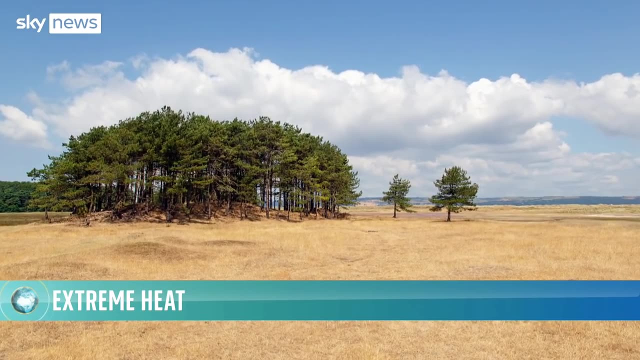 You're watching The Daily Climate Show on Sky News on today's programme. As the first ever extreme heat warning is issued in the UK, we look at how climate change is affecting temperatures. US Climate Envoy John Kerry visits the UK saying there's an urgent. 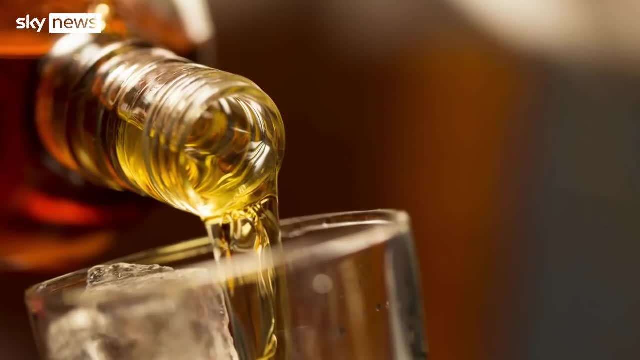 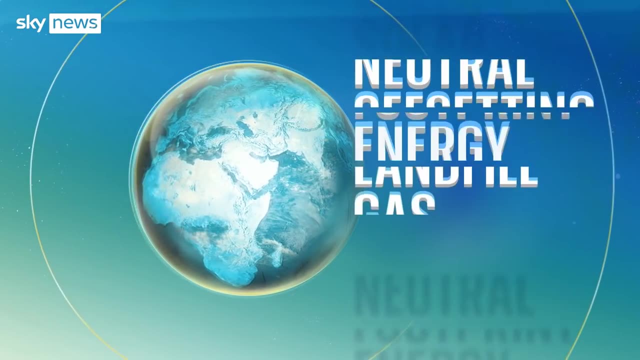 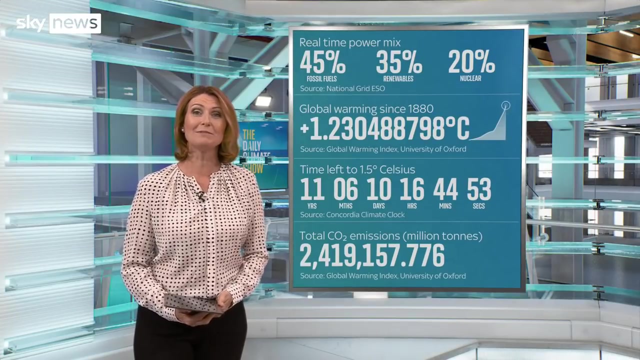 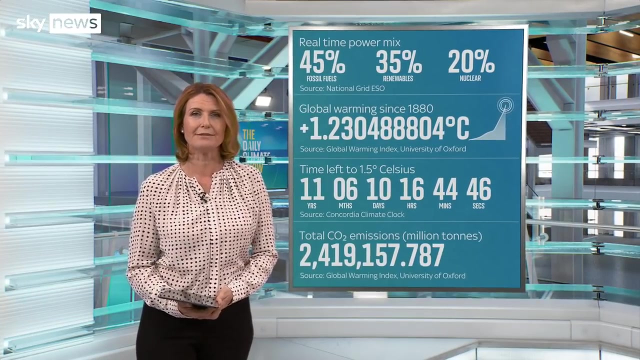 need for global climate action And find out what impact your pint has on the climate. Hello and welcome to the UK's only daily climate news show, where we track the changes happening to our world right now and meet those coming up with solutions. Well, we're starting. 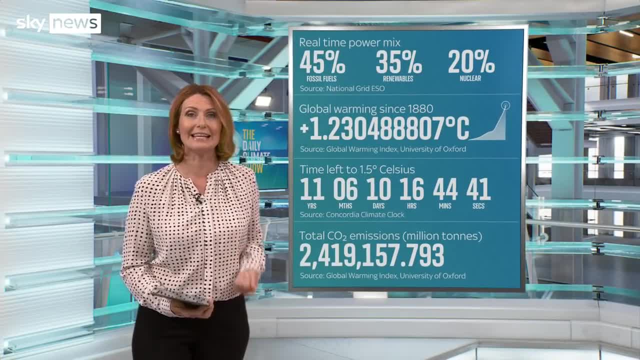 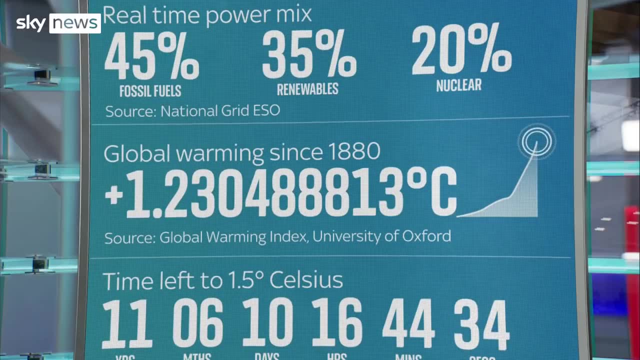 today at our data dashboard because our planet is heating up. The world is now just over 1.2 degrees warmer than it was before the industrial revolution, and that's having an impact on our weather, causing more frequent and intense droughts. We're also looking at climate change. 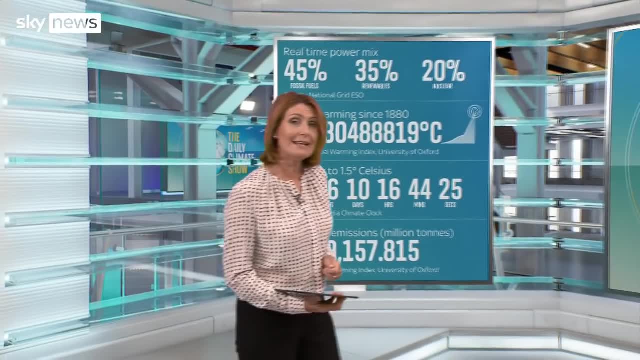 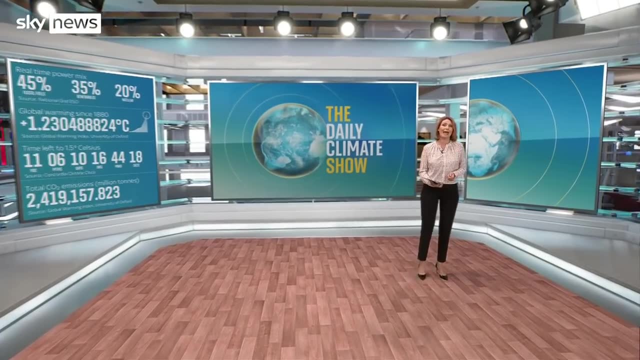 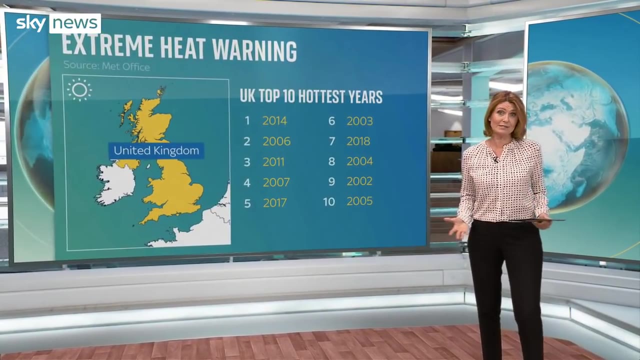 impacts wildfires, storms and rainfall. The devastating flooding in parts of Europe last week has already been blamed by some on climate change, And now here in the UK, the Met Office has issued its first ever extreme heat warning. Well, the top 10 warmest years for the UK since. 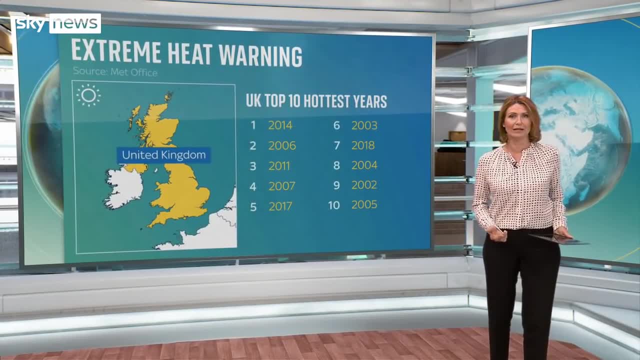 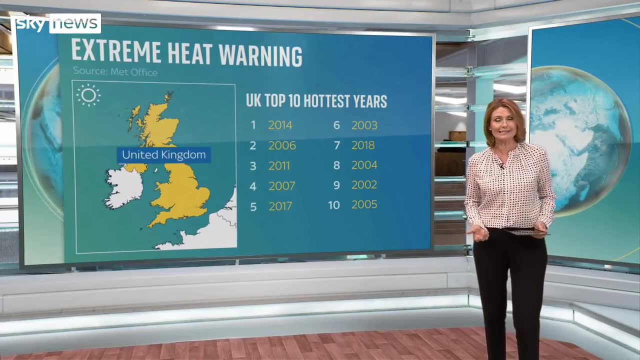 1884 have all occurred since 2002.. 2019 alone broke four records, including the warmest winter day on record and the warmest Easter day. Let's remind you of the hottest temperatures recorded in each part of the UK- In England. 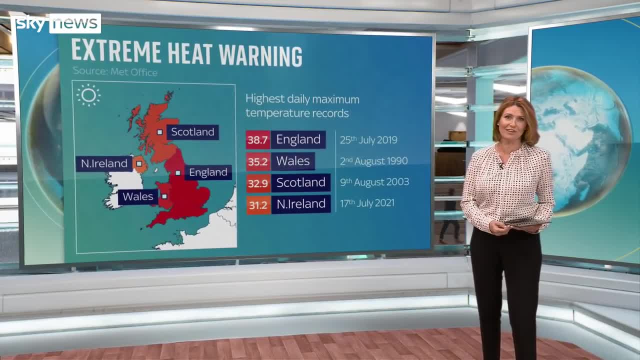 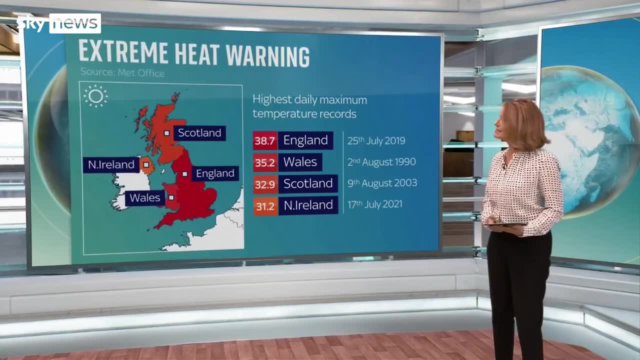 Cambridge Botanic Gardens hit 38.7 degrees in July 2019.. The record high in Wales was 35.2 degrees in 1990.. Scotland hit nearly 33 degrees in August 2003.. And a record temperature was set in Northern. 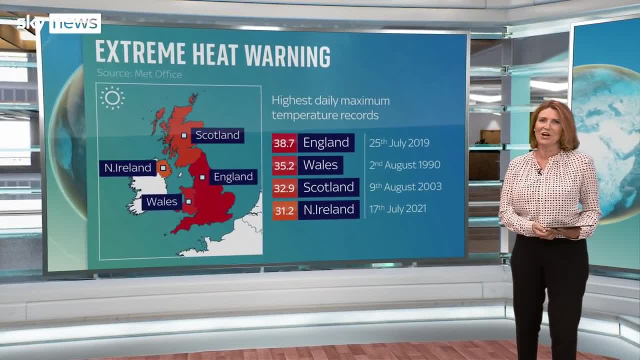 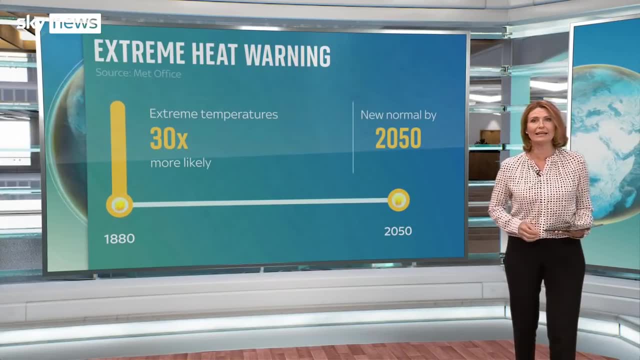 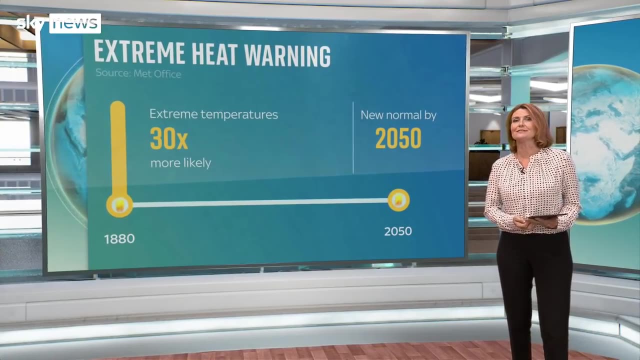 Ireland this weekend, with Ballywhattiecock in County Down reaching 31.2 degrees Celsius. Well, extreme summer temperatures are now 30 times more likely than in pre-industrial times. The latest Met Office projections of future UK climate change suggest summer temperatures now classed as heat. 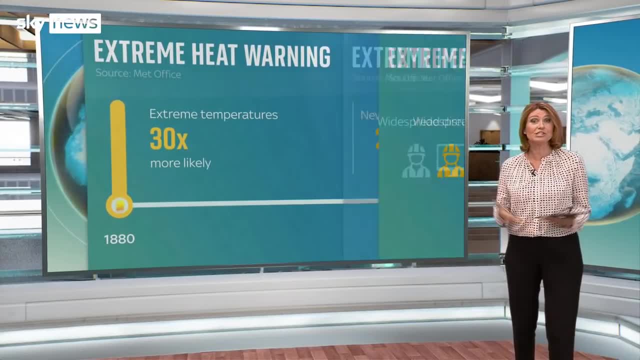 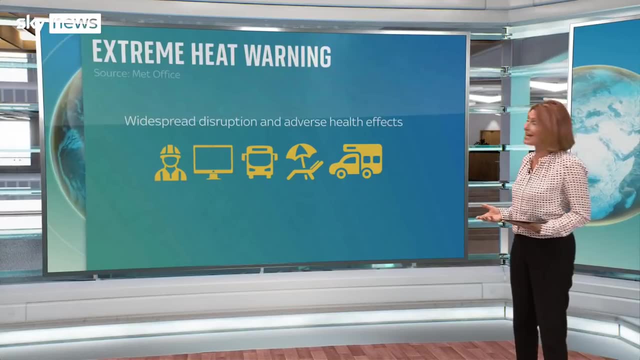 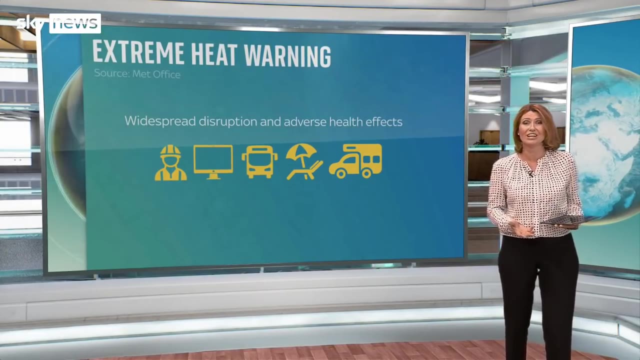 waves could be the norm by the 2050s, which is the context to the new extreme heat warning And it's issued to highlight potential widespread disruption and adverse health effects. It means changes to working practice, says might be needed. Heat sensitive systems and equipment could fail. 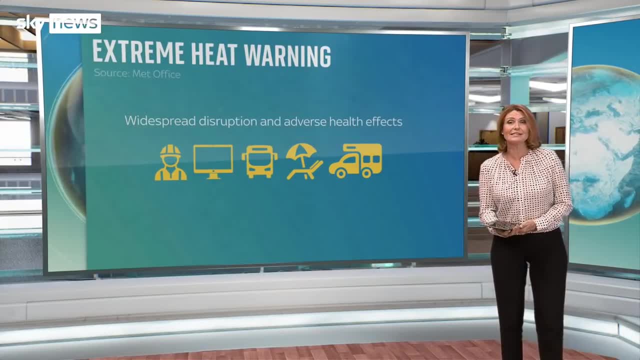 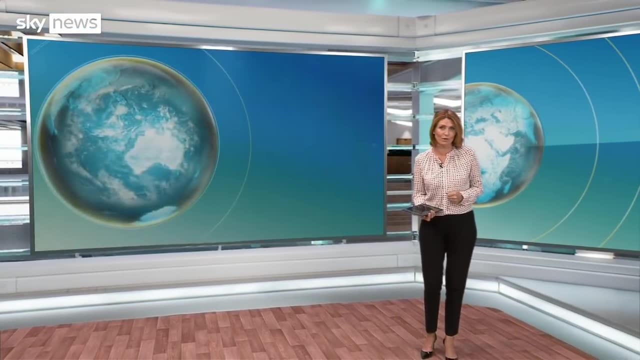 Transport could be disrupted and more people are more likely to visit coastal areas and rivers and lakes, which leads to risk of water safety incidents, While our science correspondent, Thomas More, is in South Oxford for us. Thomas, is the UK prepared for this? 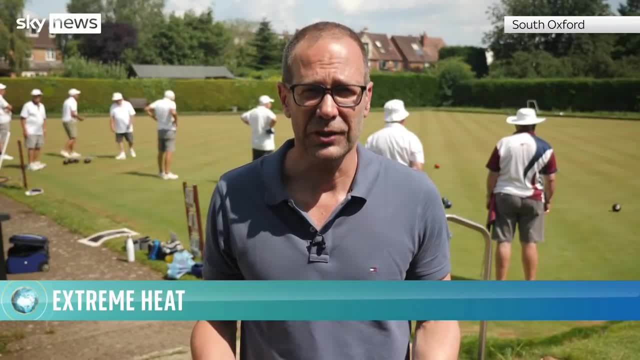 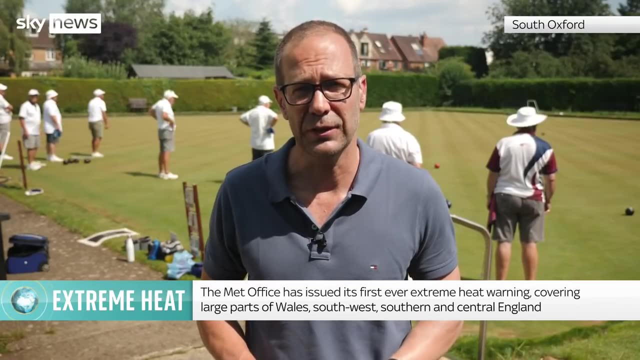 In a word: no, Jane. I think the problem is that people just aren't aware enough of what heat can do. Two and a half thousand people died last summer as a direct consequence of heat and and that is likely to increase with climate change. 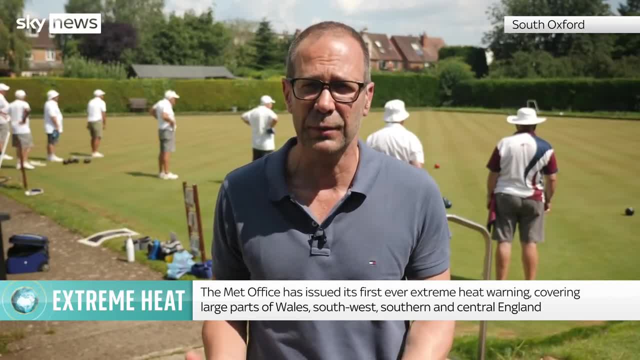 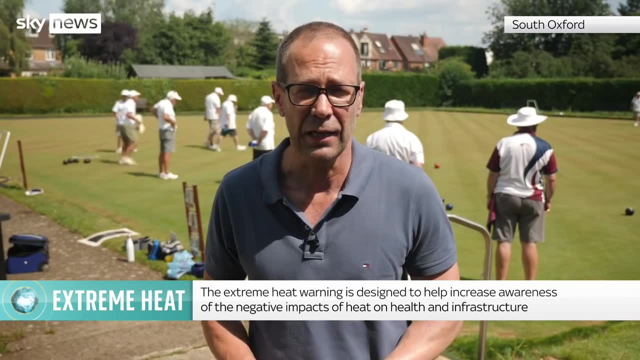 And the government has a heatwave plan, but the problem is that the alert system isn't being triggered early enough. Many people are ending up in hospital and even dying without an alert going out. Now, part of that is about behaviour change, and here at South Oxford Bowls Club, 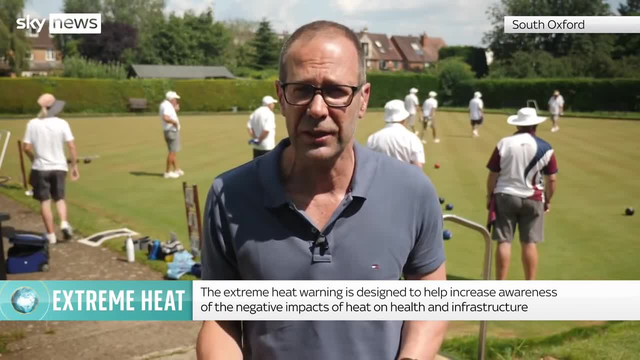 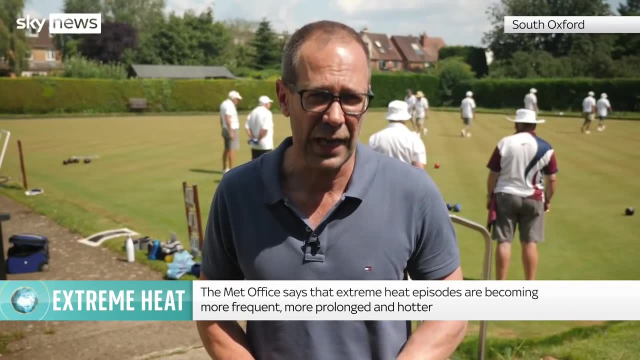 they've just taken a break in the shade for some cold drinks, but it's also about starting work earlier in the day when it's cooler. But primarily it is about housing, and 20% of people live in houses that overheat And they can get no relief from these high temperatures. 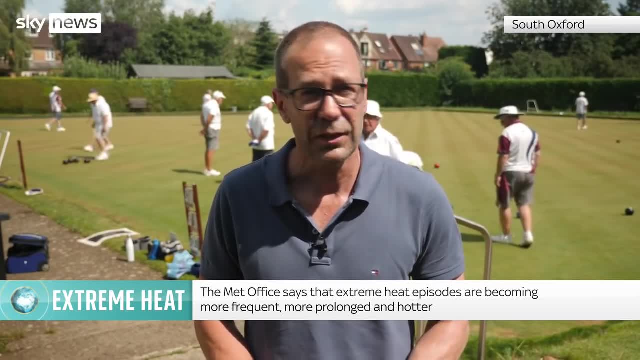 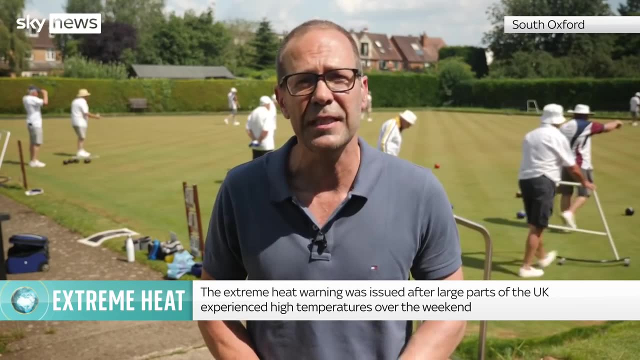 and that is a fundamental problem with the design of our buildings at the moment. There is also the infrastructure: Railways buckle under the heat Bridges too, And this is a problem that needs to be resolved because, as I say, climate is only going to get worse. 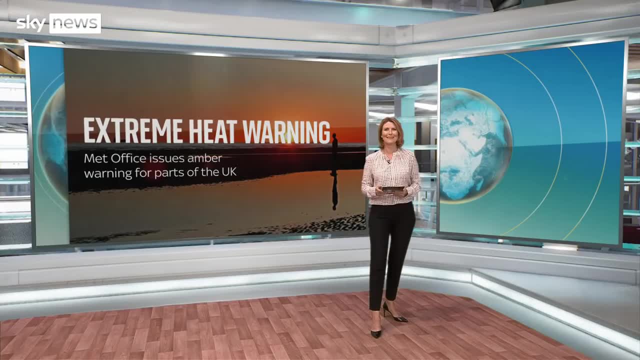 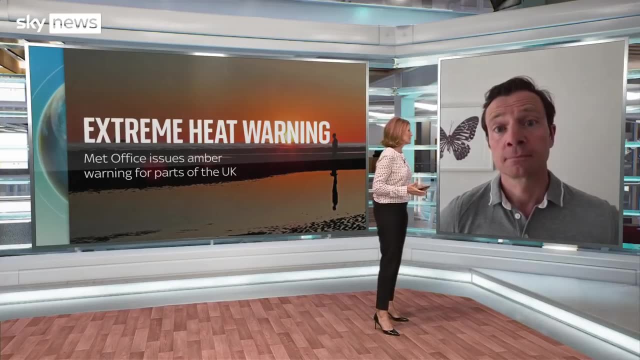 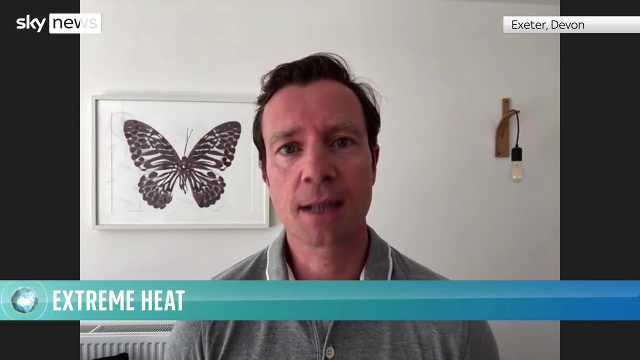 Thomas, thanks very much. Well, let's bring in Alex Deakin, meteorologist at the Met Office. Alex, can you explain why these heat warnings might become more commonplace Or frequent? Well, climate change is the simple answer to that. 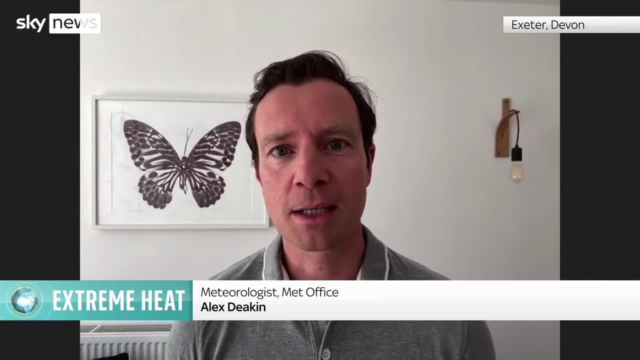 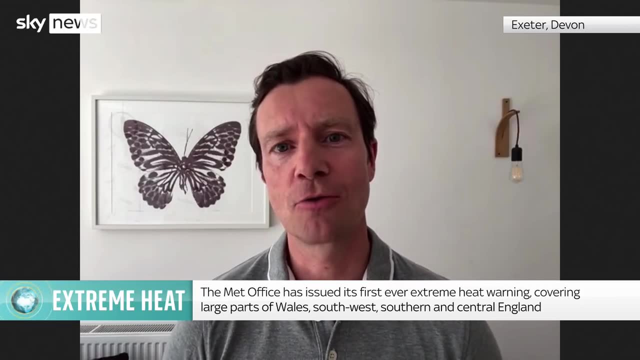 The climate is warming up. We know that across the planet, but also across the UK. We've seen that because we've got very detailed information going back well over 100 years, In some instances several hundred years, of the temperature in the UK. 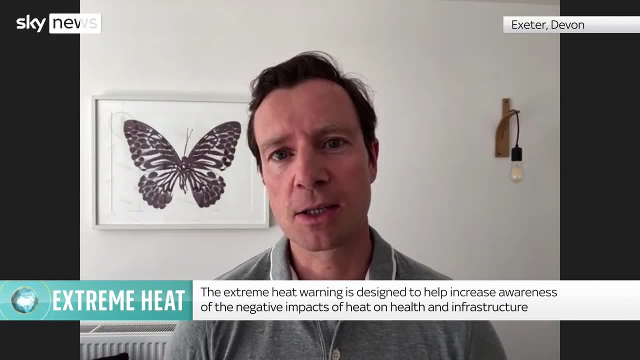 We can see it's been rising and it's more likely over the next few years, few decades, that we're going to see more extremes. All the computer models suggest that, And not only are we just seeing a shift, so that the average temperature has increased. 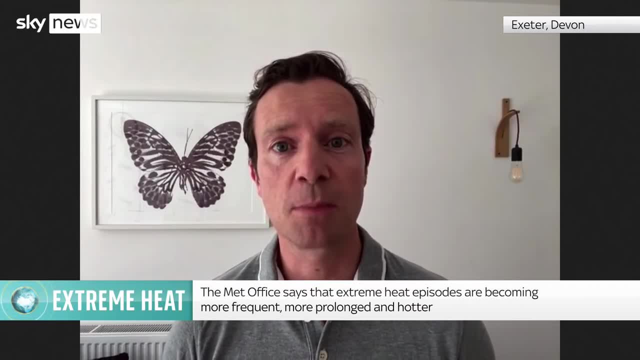 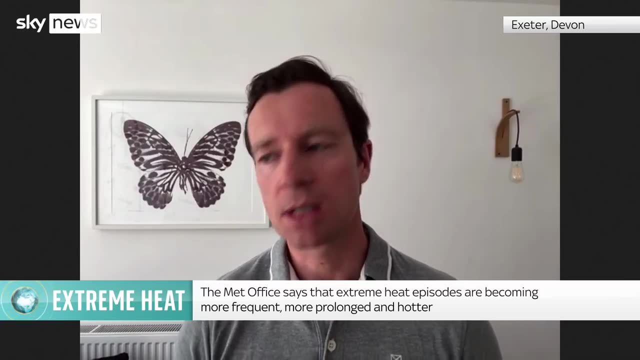 we are just seeing more frequent episodes of these extreme temperatures, So we're only going to see more of them in the future, And the peak of the extreme is also likely to rise. So when we see the top end of the extreme, it's likely just to get pushed, pushed further and further. 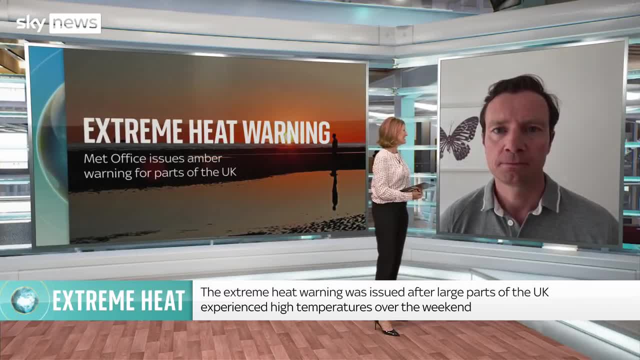 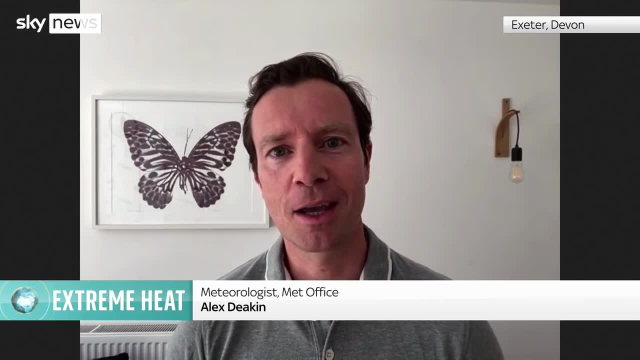 So more records will be broken. I mean, theoretically, how hot could it get? Well, that's a tricky one to answer. Obviously, the UK is an island surrounded by cooling seas, And it's not really a question about how hot it's going to get. 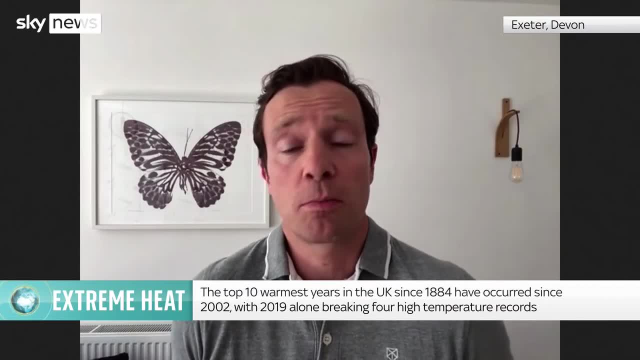 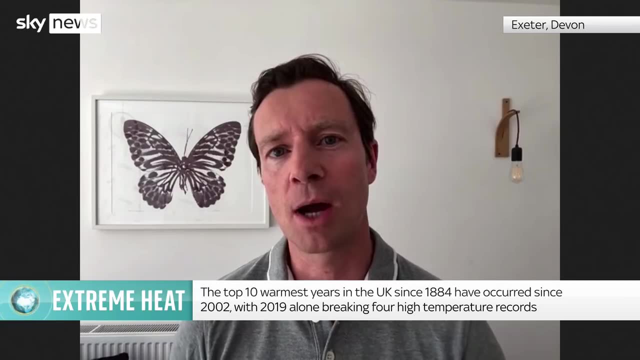 in terms of, you know, compared to other places around the planet. It's what we can cope with in this country And it's about managing expectations and getting the infrastructure right so that we can cope with the rising temperatures. We are expected to see extremes be pushed and pushed. 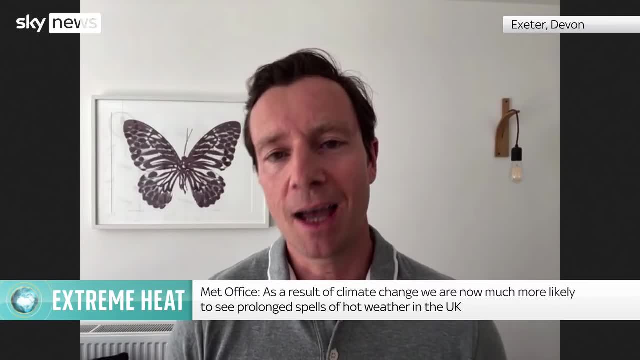 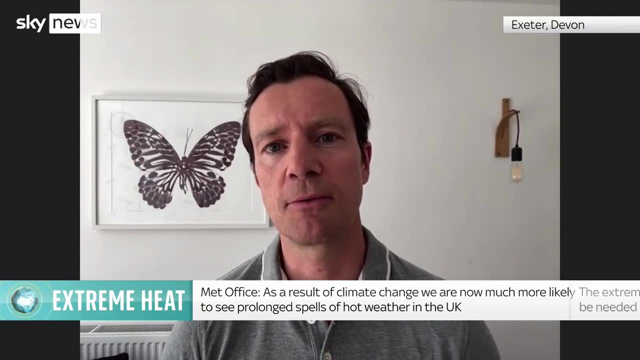 further and further, But it's more about that kind of just general seeing more of these extreme weather events. So it's not just about the temperatures, It's about more extreme rainfall as well, So we're more likely to see floods. It's all about the extremes and the ability. 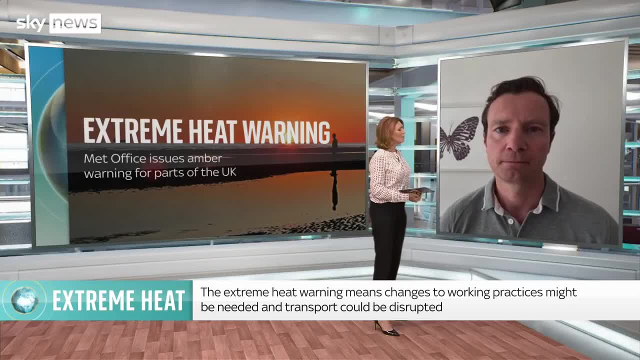 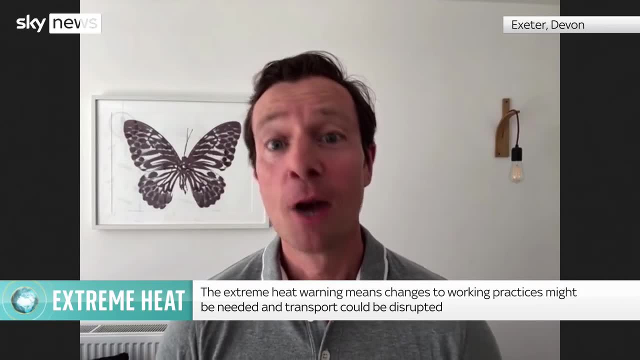 for the UK in particular, to cope. What about those, Alex, who will just say, well, this is just the weather. I remember hot summers from my childhood. Well, the answer to that is they're simply becoming more and more frequent. 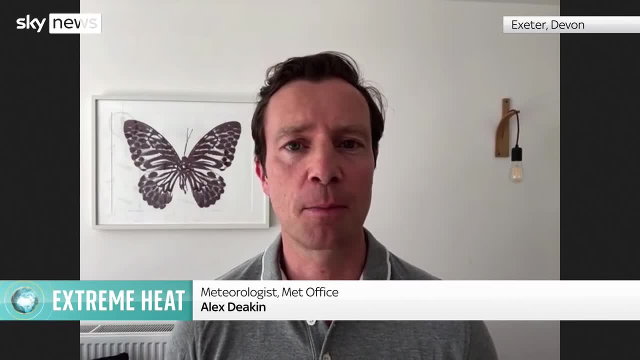 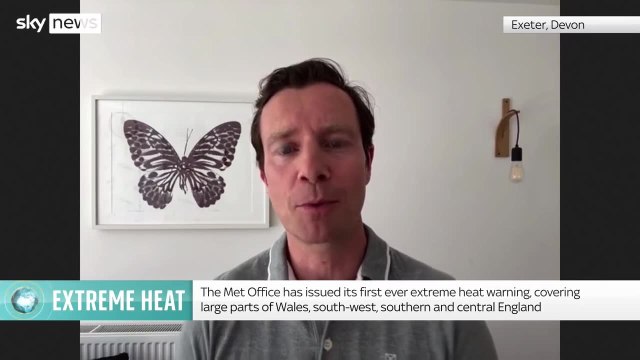 And we've got all the statistics to back that up. For example, 2018, the joint hottest summer on record, joined with 1976.. People do often remember that one and cite that one, But that was followed by 2019.. 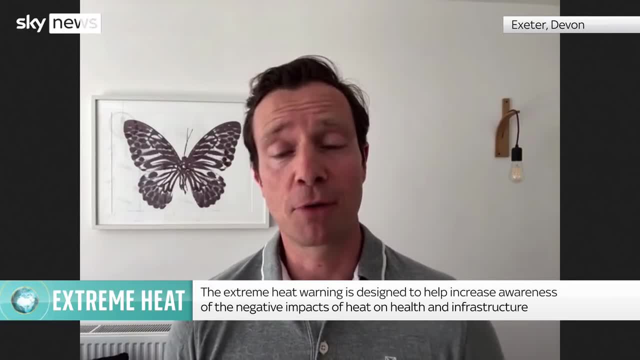 So what's the next step? So in 2019, where we saw the highest temperature ever recorded in the UK, and then 2020, which was the third warmest year on record in a series going back well over 100 years, The statistics are clear. 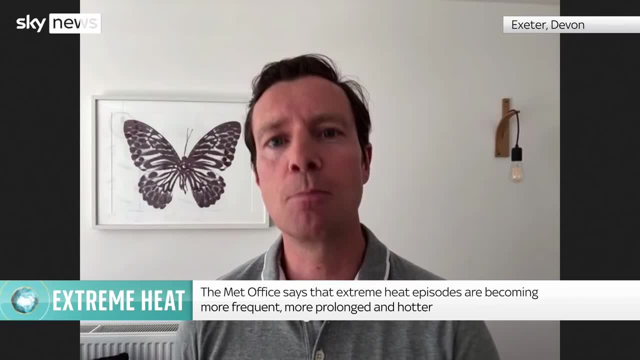 Everything is pointing to the fact that things are getting hotter and we're seeing more and more of these extreme events. All the computer models suggest that by 2050, the summer of 2018 will be a one in two year event, So it'll be a fairly typical summer. 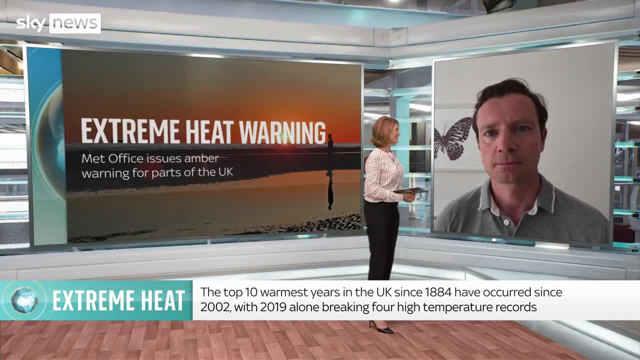 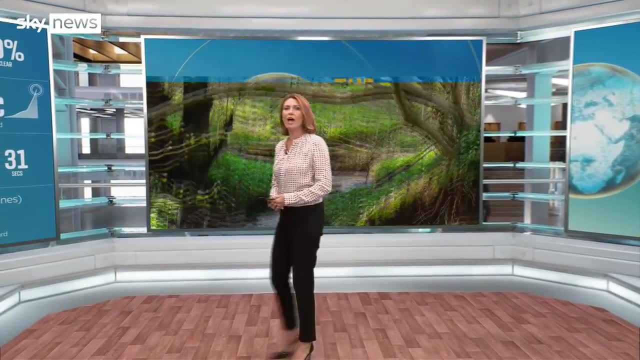 And that was, as I say, the joint hottest on record overall. Alex Deacon, thanks very much. Well, in today's other climate news, the government is being urged to create 100,000 hectares of wetlands in the UK to help combat the climate crisis. 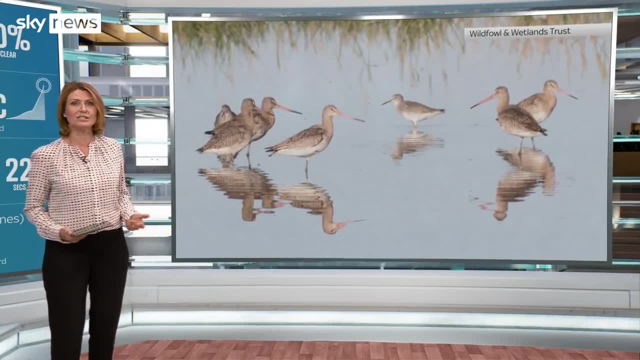 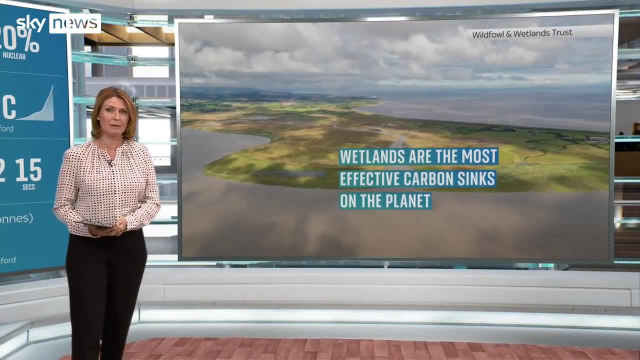 The Wildfowl and Wetlands Trust says that wetlands are vital as they store carbon, reduce flooding and help biodiversity. New research by the charity found that more than three quarters of people in Britain think that there should be more investment in natural solutions. 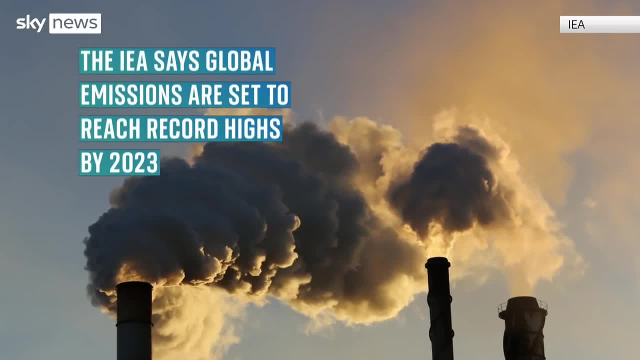 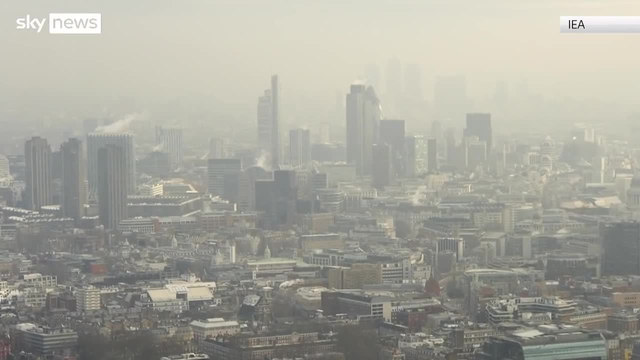 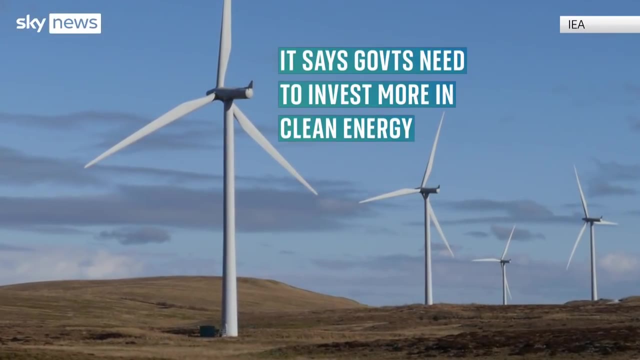 The International Energy Agency is warning that global emissions are set to soar as economies recover from the pandemic. The agency estimates governments around the world have only allocated 2% of their recovery fund to clean energy measures. It says global clean energy investments need to increase. 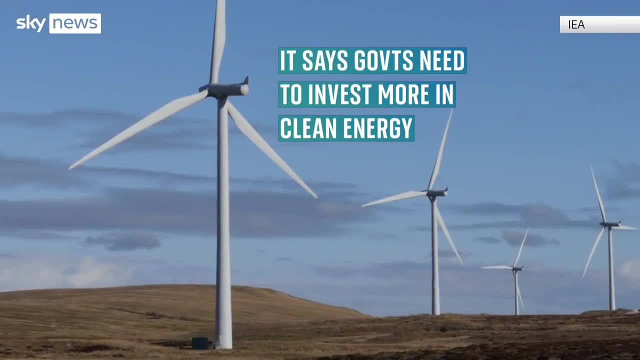 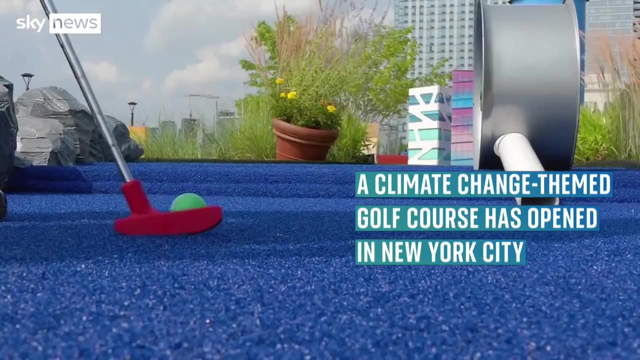 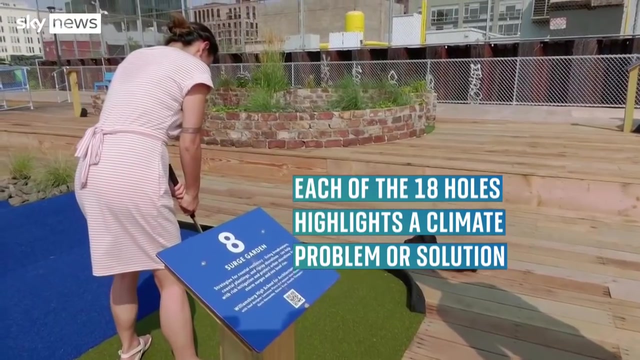 by around two thirds to prevent emissions reaching record levels by 2023.. And a mini golf course has opened in New York City which aims to teach players about climate change. Local artists and non-profit groups have designed the 18 holes at Putting Green to highlight environmental issues and solutions. 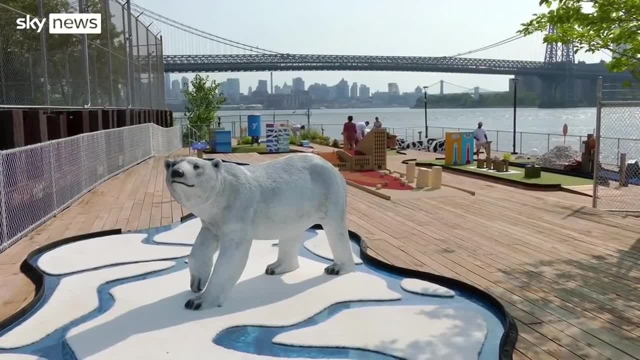 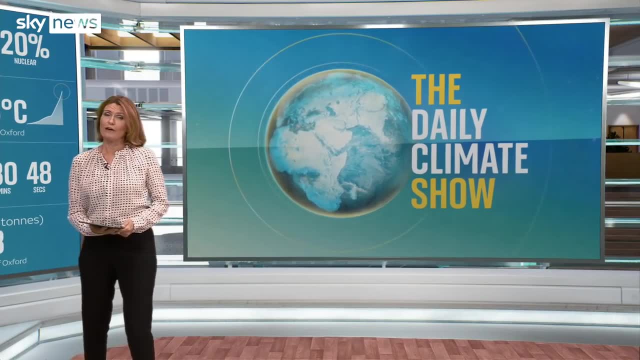 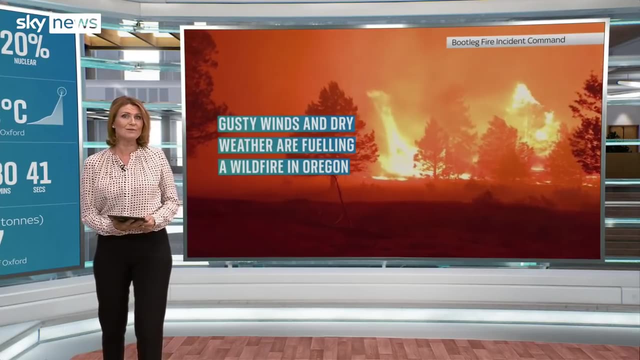 Players can find out more about wind energy emissions and the effects of melting ice caps by reading information on placards whilst they putt To the US now, where officials in Oregon are asking for help to contain a massive wildfire in the state, The Bootleg Fire has grown to 537 square miles. 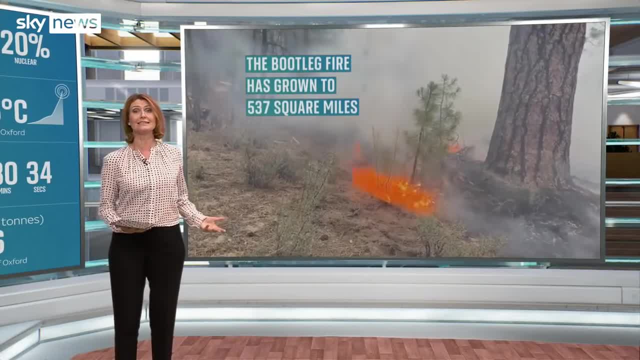 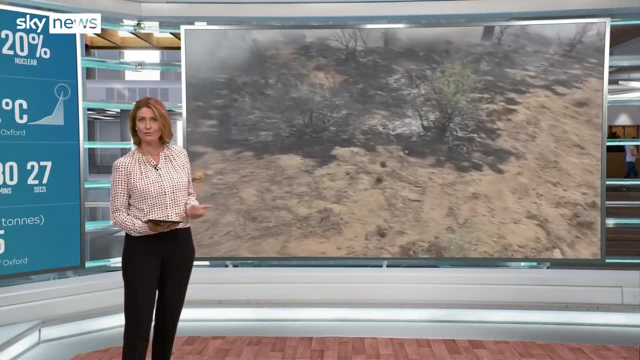 Due to gusty winds and dry hot weather, which is expected to continue over the coming days. it's one of more than 80 wildfires to have broken out across the Western United States, forcing thousands to flee their homes. Scientists say climate change has made the West much warmer and drier. 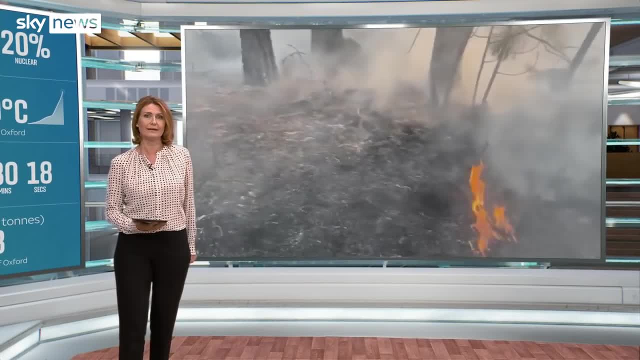 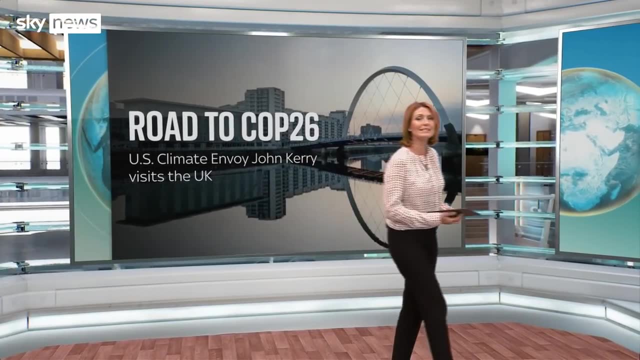 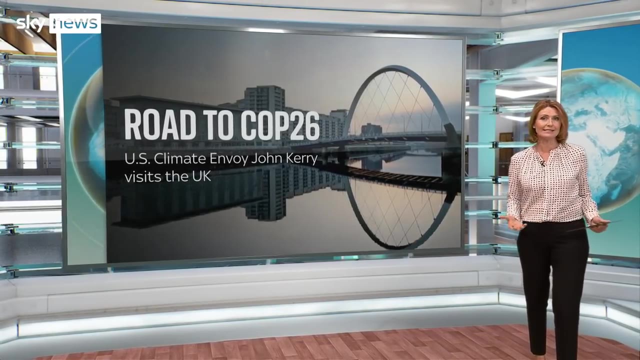 and will continue to make weather more extreme and wildfires more frequent. Well, this comes as there are just over 100 days to go until the most important climate summit in years, COP26.. The conference will be held in Glasgow in November, bringing together heads of state, business leaders, scientists and campaigners. 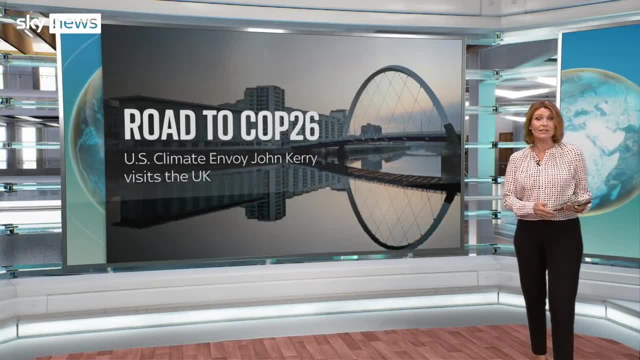 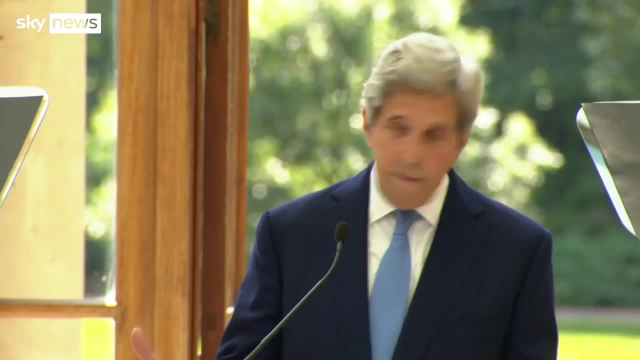 And ahead of the meeting, the US climate envoy, John Kerry is in the UK. Earlier he visited Kew Gardens in London and spoke about the urgent need for global climate action, Even if everyone did what they said they would do in Paris. 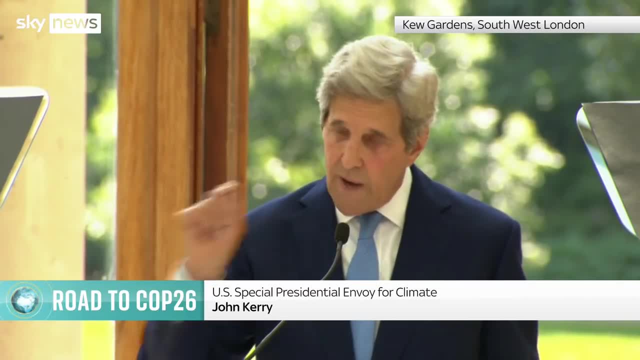 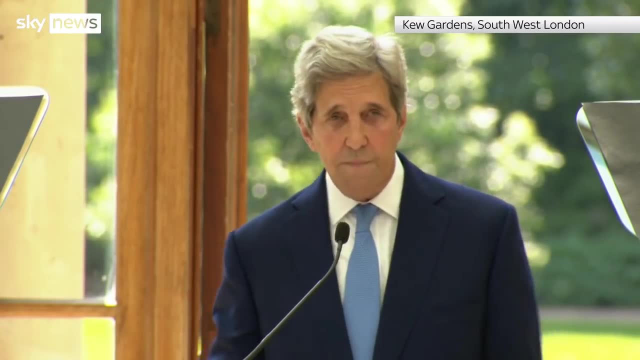 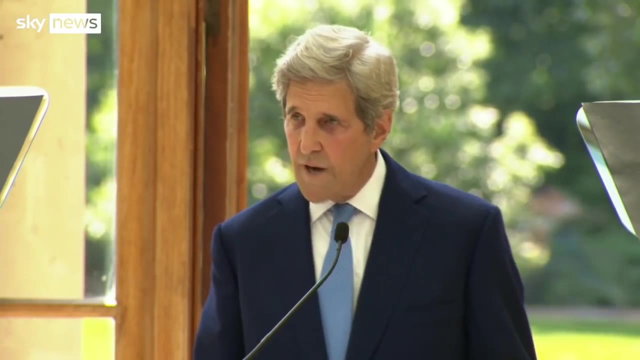 the temperature of this planet will still rise by upwards of 2.5 or 3 degrees centigrade. We're already seeing dramatic consequences with 1.2 degrees. Imagine the doubling. To contemplate doubling that is to invite catastrophe. Our climate correspondent, Hannah Thomas-Peter. 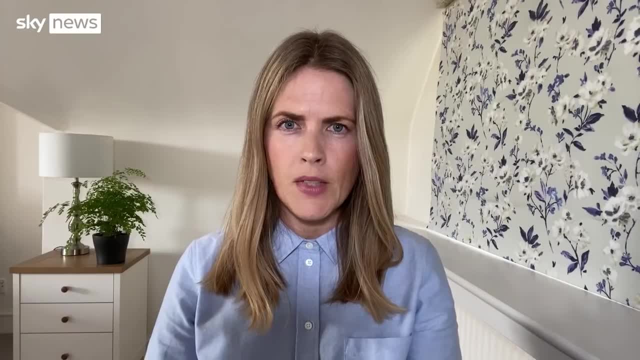 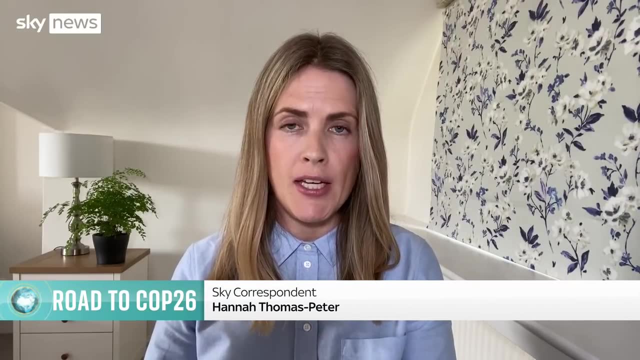 was listening to that speech and has the latest. That was as strong a speech as I've heard from Special Envoy John Kerry on the subject of climate change, a speech that sounded like it was being fuelled by something that was causing so much frustration and anger. 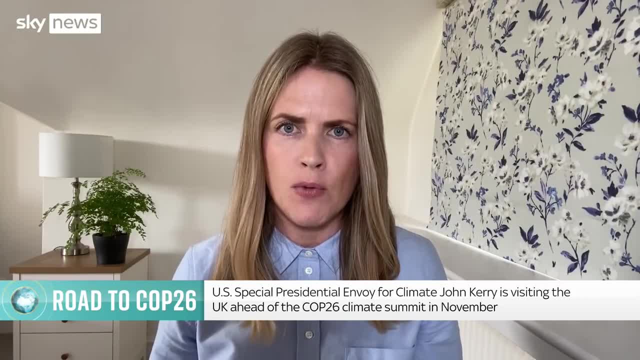 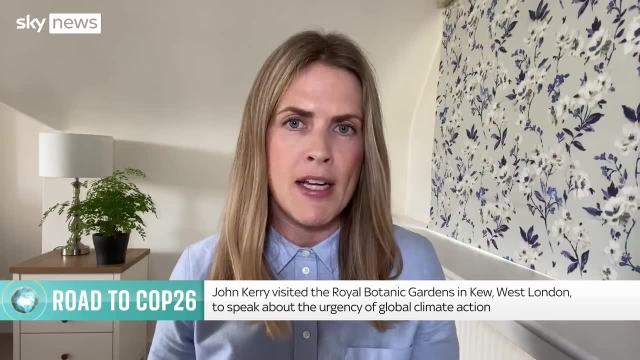 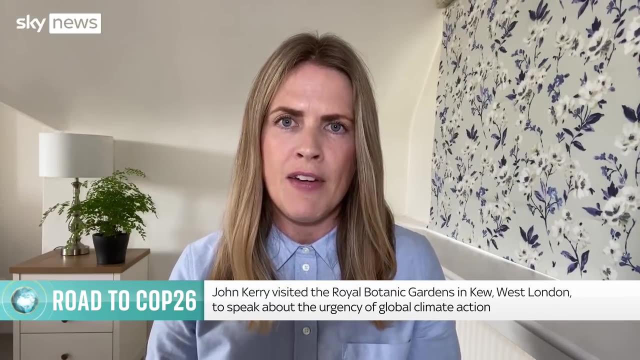 Definitely frustration that we are now in the defining decade of action when it comes to international consensus and commitments to reduce carbon emissions and that we have no alternative but to get this right, Because he painted a very scary picture of an increasingly unlivable, unstable world if it continues to warm. 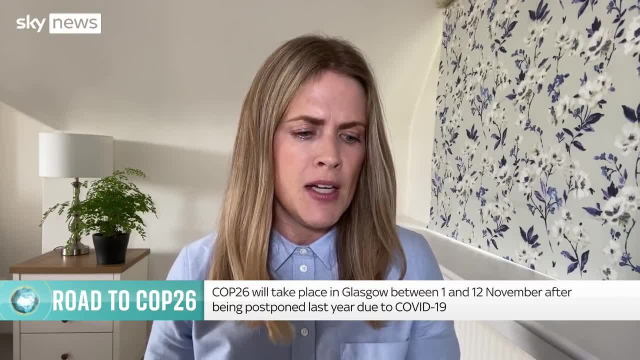 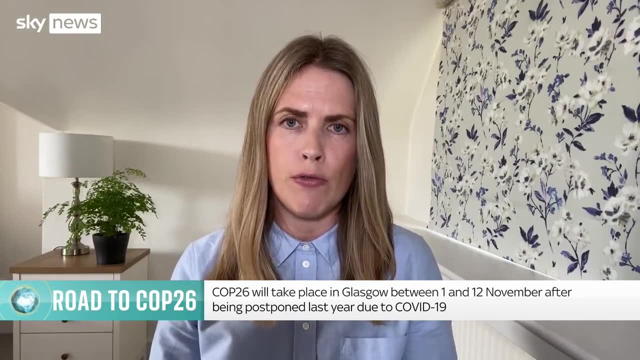 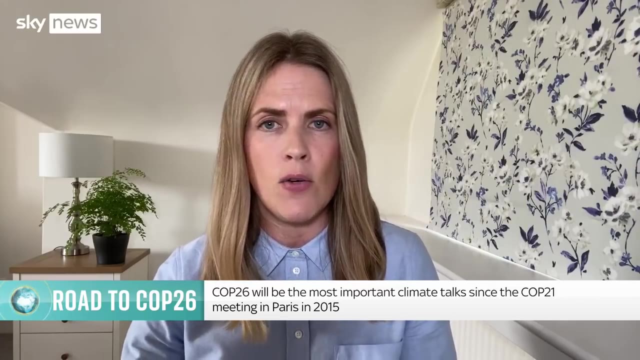 He called climate change the test of our time, an acute and as existential test as any previous, And he laboured the point that no country, rich or poor, will be spared, and then spoke about the extreme weather that we have been seeing in Western Europe. 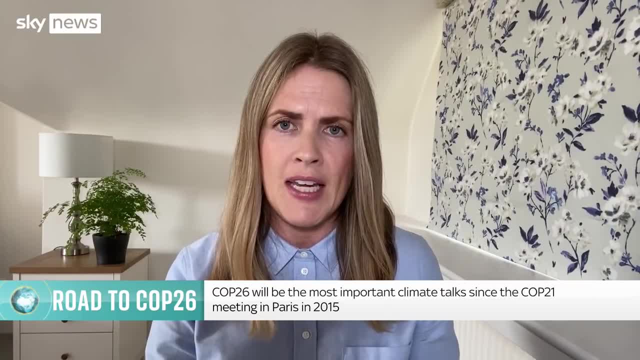 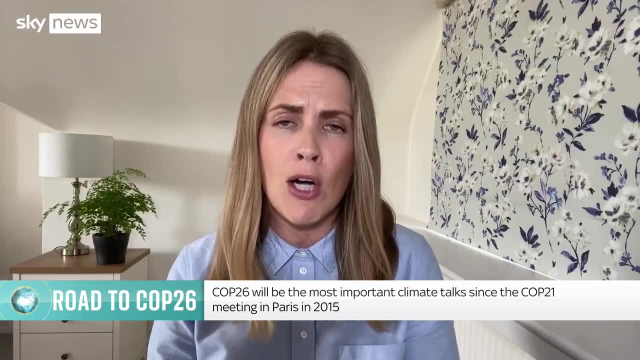 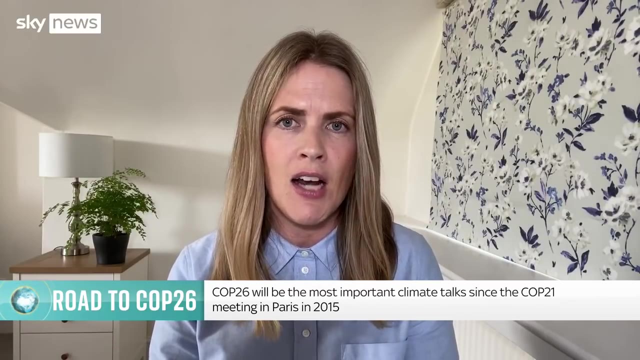 in terms of the floods and in America in terms of the heat, And it's interesting because climate scientists themselves are getting more and more confident about how closely they can link climate change to these individual extreme events. We've just spoken to NASA's senior climate adviser. 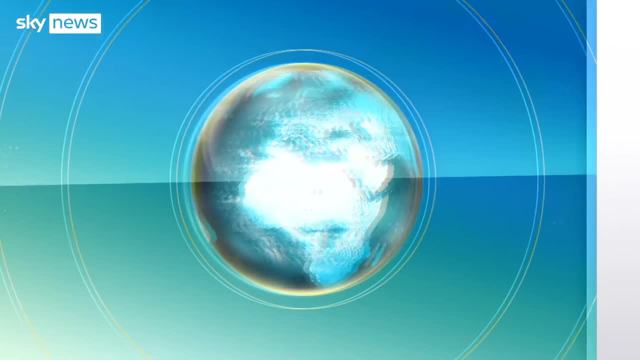 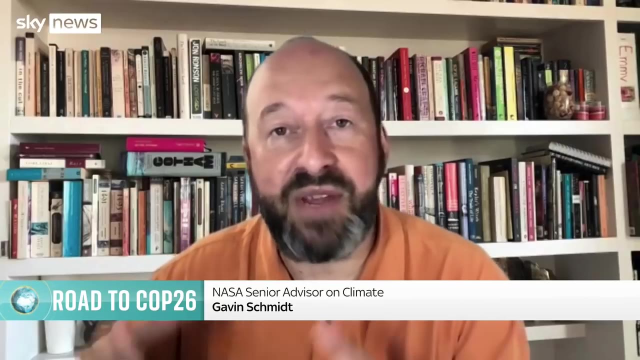 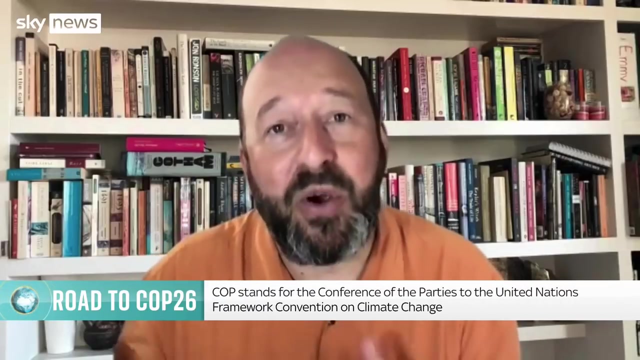 Gavin Schmidt, and this is what he had to say. When we've seen situations like in the Pacific Northwest, which blew through the records in such a dramatic fashion- you're looking at ratios like 150 times, maybe a thousand times, more likely to happen now than it would have done- at which point you can start to say: 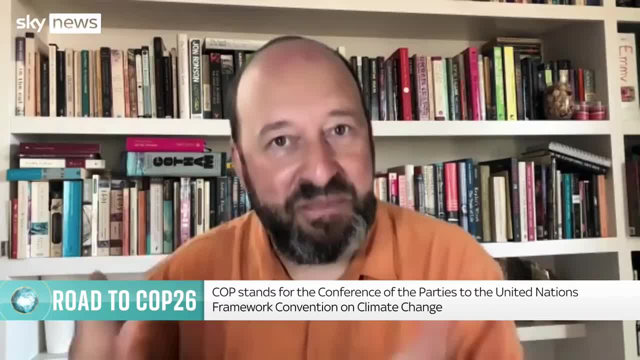 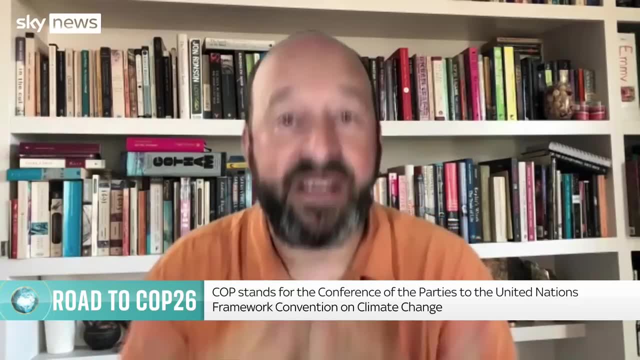 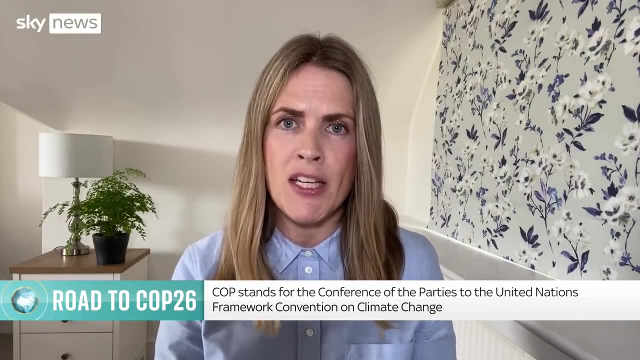 well, it would never have happened before, And so you can basically say that this event is almost 100 percent attributable to the fact that the climate has changed. And when you start to hear messages like that from NASA, when you start to hear speeches like that from John Kerry,